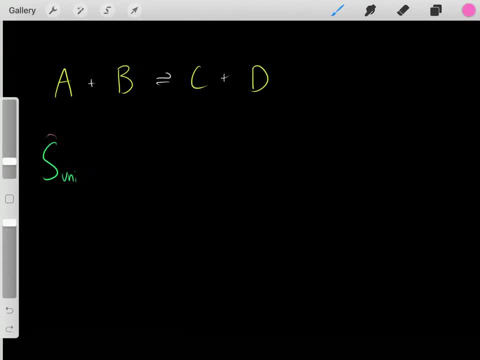 how did the entropy of the universe change? So this S term is the term for entropy. So we need to ask ourselves: how did the entropy of the universe change when this reaction occurred? And if the entropy of the universe increased when this reaction occurred, then we know it. 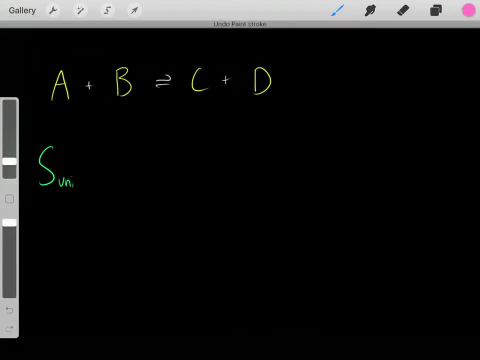 will occur spontaneously. However, if this reaction leads to the entropy of the universe decreasing, then this will not be spontaneous, And that's the only qualification, that's the only thing that's important when determining whether this reaction will occur spontaneously or not. So now you might wonder: 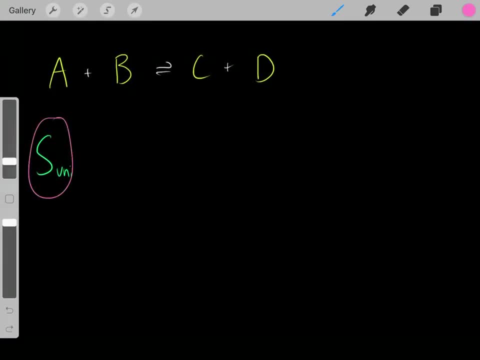 when determining if this reaction will occur spontaneously, you need to determine if the entropy of the universe increased. So how do we determine if the entropy of the universe increased? Well, what makes up the universe? Well, there are two things that make up the universe. 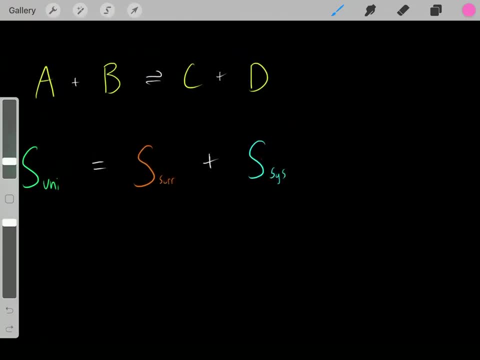 This system, this system and the surroundings and everything else in the universe. Those are the two things that make up the universe. So, again, the system is comprised of the atoms, the atoms of this chemical reaction. Those atoms make up the system. 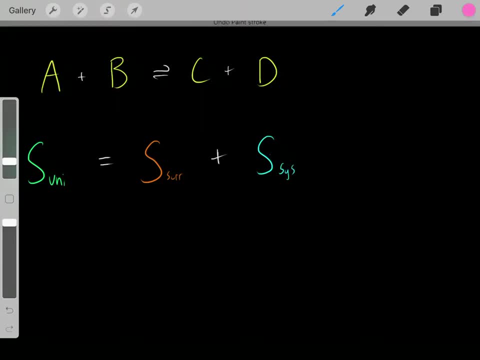 Everything else in the universe, the surroundings. everything else in the universe is again the surroundings, and it's those two things, this system and everything else in the universe, which make up the universe. So now, when determining if this reaction will occur spontaneously, 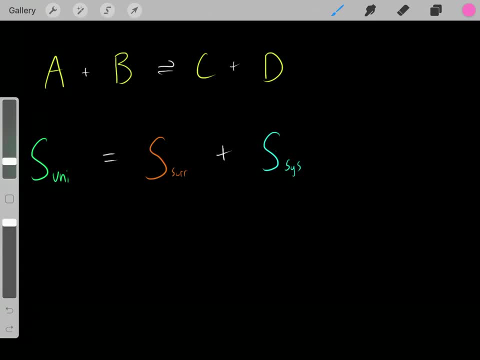 we need to determine if the entropy of the universe increased. If the entropy of the universe increased when this reaction occurred, we know this will occur spontaneously. So to determine if the entropy of the universe increased, we need to know how the entropy of the surroundings 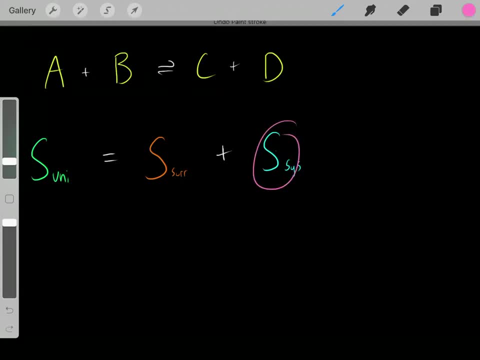 changed and we need to know how the entropy of the system changed. And if we know how those two entropy has changed, we know how the entropy of the universe changed. So, for example, when this chemical reaction occurs, how do we know if the entropy of the system increased or decreased? 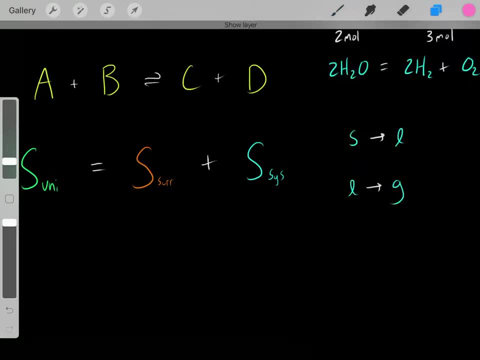 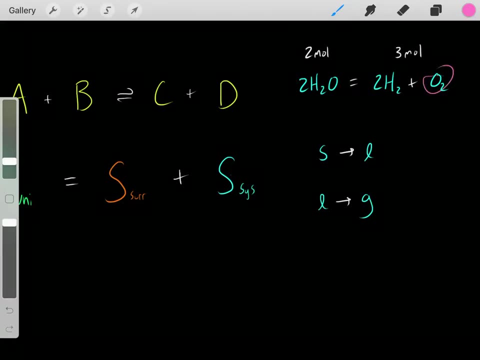 How can we determine that? Well, the rule of thumb is: first of all, let's say we had this chemical reaction where two water molecules reacted, forming two hydrogen atoms and one oxygen atom. When this chemical reaction occurred, first we had two moles of compounds, but then we went through. 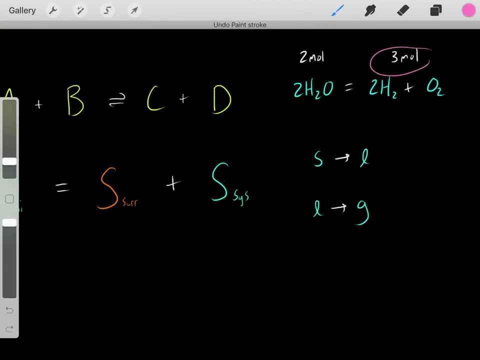 the chemical reaction. now we have three moles: Two of this guy, one of this guy, so three moles in total. So when this chemical reaction occurred, we ended up with more moles. And whenever a reaction occurs where now we have more moles, that's a reaction where the entropy of the system increased. 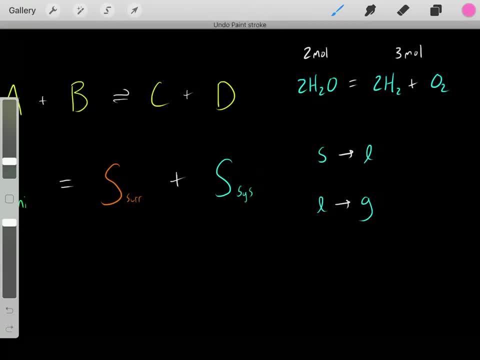 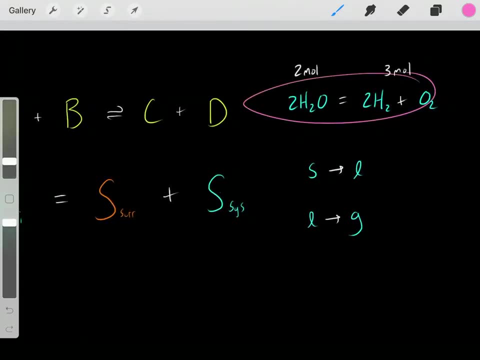 So this reaction, the entropy of the system increased, which is favorable because again that helps promote the universe increasing. So again, that's just a rule of thumb you need to be familiar with: Whenever we have a certain amount of moles, then they react. now we have 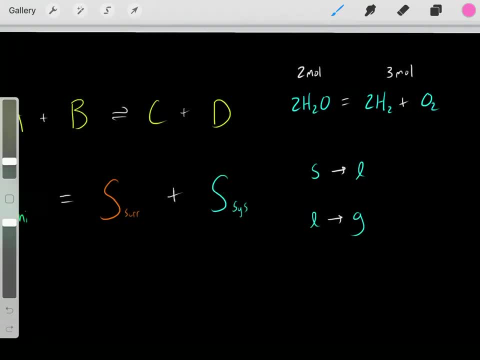 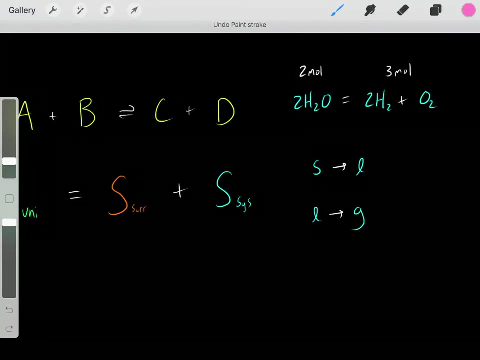 more moles, That means the entropy of the system increased. So the entropy of the system would increase. And another rule of thumb is: whenever you have a solid turning into a liquid or a liquid turning into a gas, these both represent systems that have increased entropy. For example, maybe we have 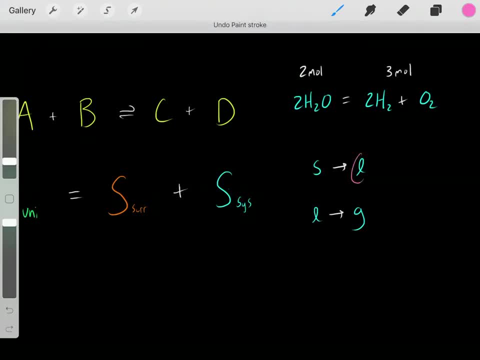 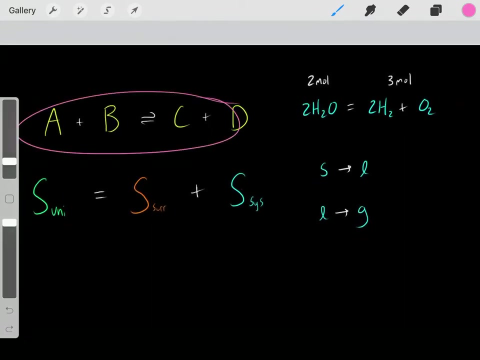 water melt, or we have ice melting into water, the entropy of the system increased. Or maybe we have water evaporating into gas, the system of this system increased. So that's a rule of thumb. So again, whenever we're looking at a reaction, those are the two things. you need to be familiar. 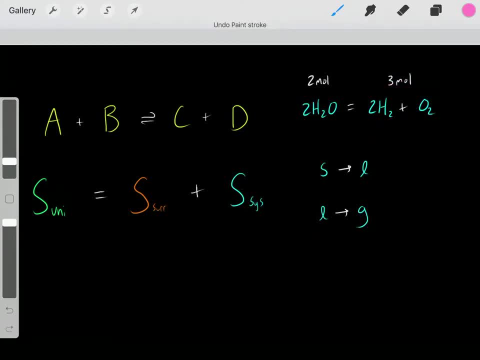 with How the phases are changing and if there's more moles And if the products have more moles, then we know the entropy of the system increased. However, maybe we had the opposite, Maybe we had four moles on this side and maybe we had two moles on this side. Then, in this situation, 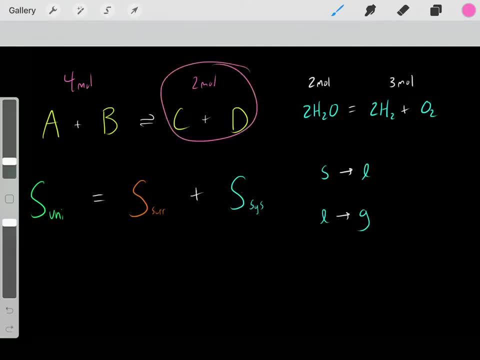 the entropy of the system decreased. We had fewer moles in our product, So in this system the entropy decreased. So for determining how the entropy of the system changed, these are the things you need to be familiar with. However, how do we know the entropy of? 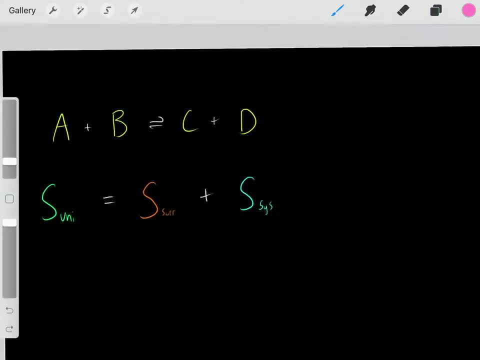 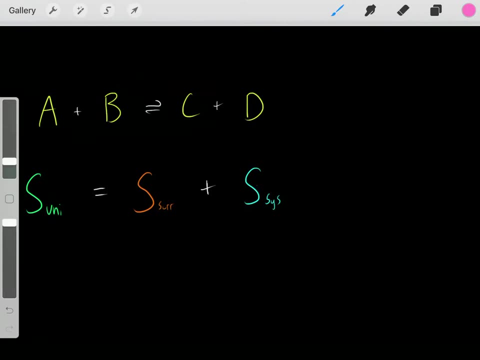 the surroundings increased Because, again, that's also important. So how do we know? the entropy of the surroundings increased? Well, this is actually very simple: If we have an exothermic reaction. so this reaction reacts and it releases heat. It releases heat as a product. 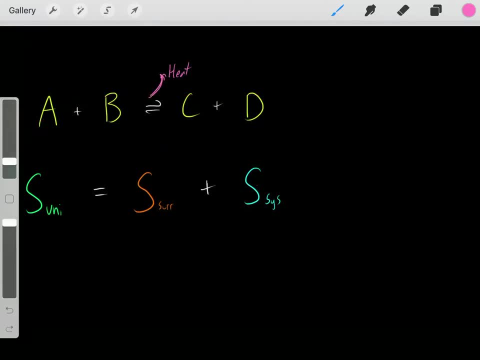 then this is an exothermic reaction And therefore this heat that's released to the surroundings increases the entropy of the surroundings. So pretty straightforward, If the reaction is exothermic, then we know the entropy of the surroundings increased. So again, that's. 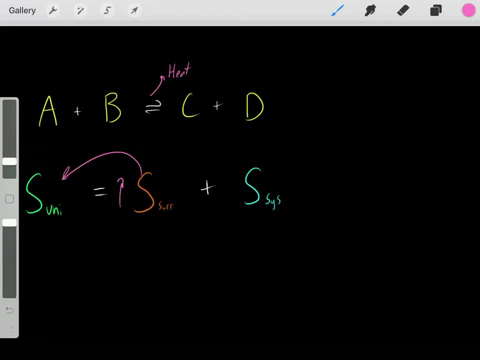 favorable because if the entropy of the surroundings increased, that promotes the entropy of the universe increasing, And again, so pretty straightforward. And if we have an endothermic reaction, if this reaction required heat and it took heat from the surroundings. 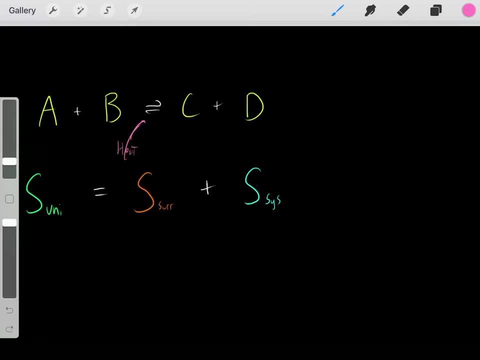 then in this situation the entropy of the surroundings decreased because it took that heat from the surroundings. So now the surroundings have the heat from the surroundings, less heat. so now the entropy of the surroundings decreased, which is unfavorable because that promotes the entropy of the universe decreasing. So those are the two terms you need to be familiar. 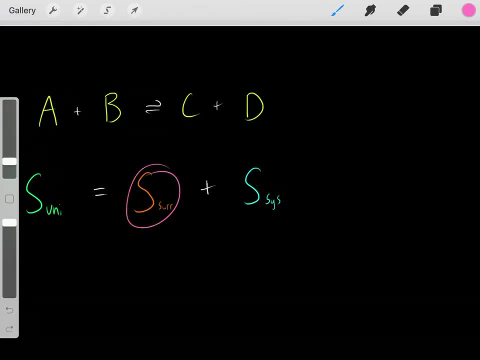 with how the entropy of the system changed and how the entropy of the surroundings changed. But realize you need to know both of them to know the entropy of the universe changed or increased or not. For example, maybe we had two moles on the reactants and maybe four. 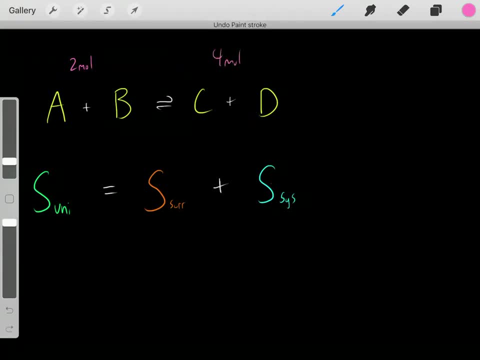 moles on the products. So therefore, we know that entropy of the system increased In this reaction. the entropy of the system increased, So does that mean the entropy of the universe increased and this reaction will occur spontaneously? Well, we also need to know how the entropy of 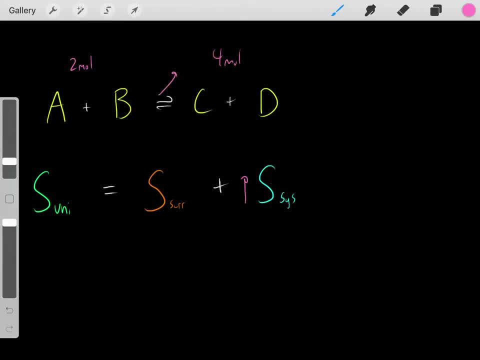 the surroundings changed. For example, if this was an exothermic reaction that released heat and therefore the entropy of the surroundings increased, then we know the entropy of the system increased, the entropy of the surroundings increased, so therefore the entropy of the universe must have increased. So therefore this reaction must have been spontaneous. 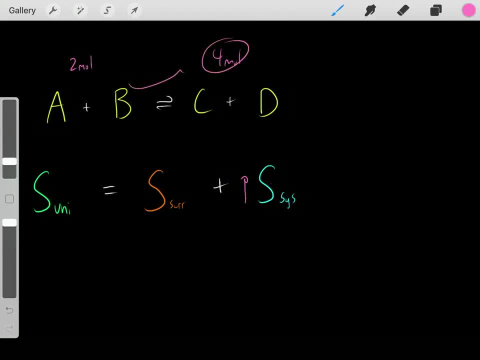 However, maybe the entropy of the system increased so we created more moles. but maybe the entropy of the system increased so we created more moles. maybe this reaction was endothermic, Maybe it required heat, So in this situation, the entropy 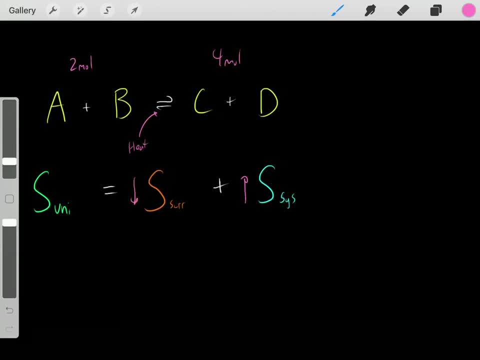 of the surroundings decreased. So this happens: How do we know if the entropy of the universe increased or not? We know the entropy of the system increased, but we know the entropy of the surroundings decreased. So how do we know overall, how the entropy of the universe increased? 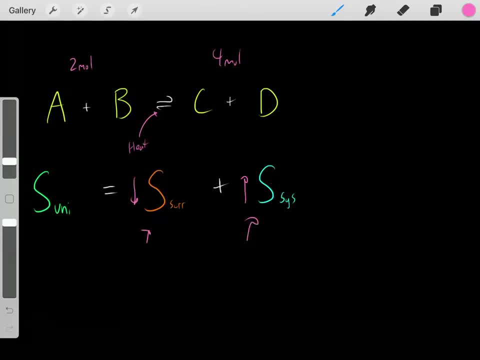 Well, again, we need to know the magnitudes, We need to know the numerical magnitudes and we can see which one is greater. Whichever one is greater has the biggest impact on the entropy of the universe. So let's do some examples to really clarify what's going on. 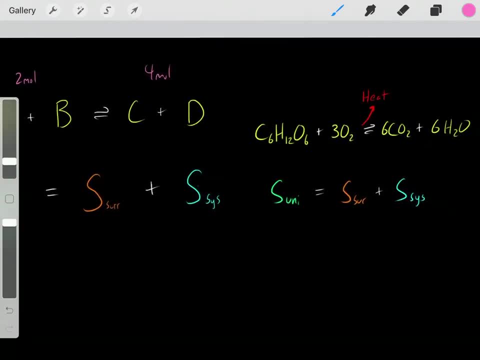 So let's say we had this chemical reaction. where again, with this chemical reaction, is this chemical reaction spontaneous? Does the entropy of the universe increase when this chemical reaction occurs? Well, first of all, let's see, We have 4 moles here and we have 12. 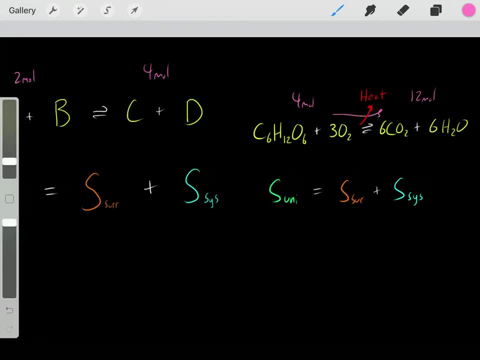 moles here. So we know we have more moles in our product. so therefore we know the entropy of the system increased. The entropy of the system increased, So we know that's favorable. but what about the entropy of the surroundings? Well, we know it released heat, It released heat. so therefore, whenever the 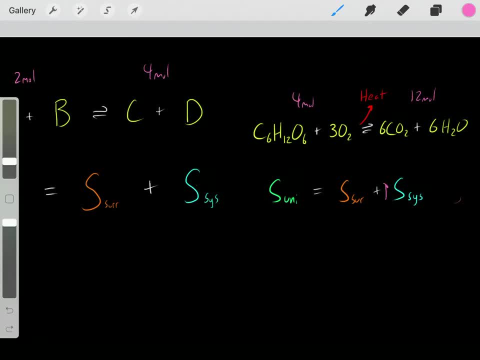 surroundings gain heat, they increase in entropy. So therefore, because this is exothermic, we know the entropy of the surroundings also increased. So therefore we know this has to be spontaneous. The entropy of the universe had to increase, so therefore we know this is a spontaneous reaction. 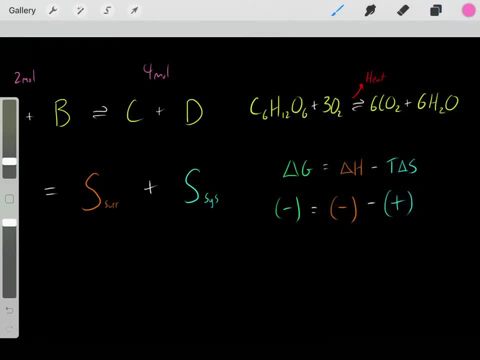 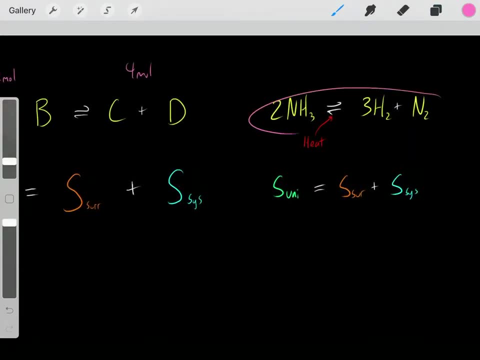 This reaction will occur spontaneously. But let's say we had this chemical or let's say we had another chemical reaction. So again, is this reaction spontaneous. Well, again, we went from 2 moles to 4 moles. So the system: 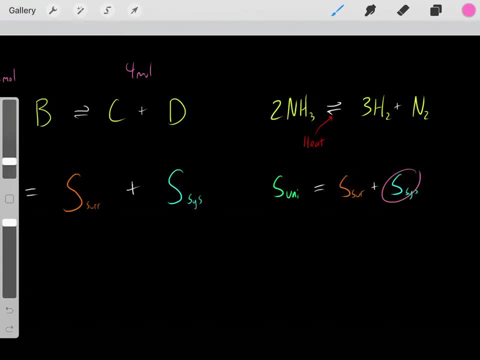 increased in the number of moles, so therefore the entropy of the system increased. The entropy of the system increased, But we know this is an endothermic reaction. It required heat, so it took heat from the surroundings. so we know the entropy of the surroundings decreased. So now how do we? 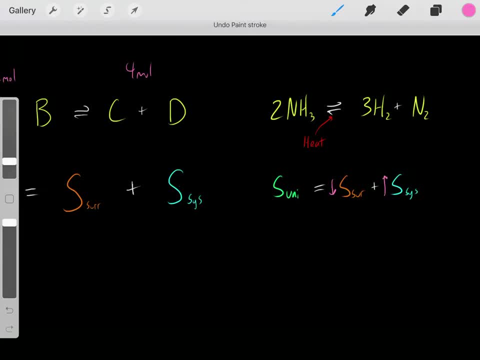 know this reaction is spontaneous. Well, we need to know the magnitudes, We need to know which of these magnitudes was greater and which of these magnitudes was less. So we need to know the immensity which has the bigger impact on entropy of the universe. But once we can determine that, 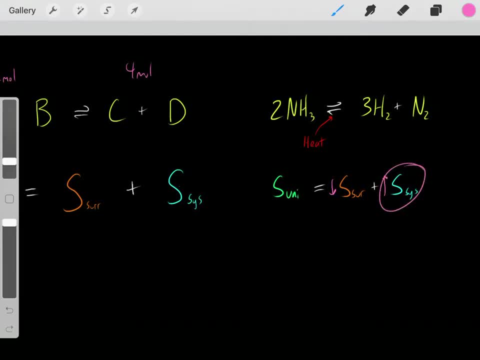 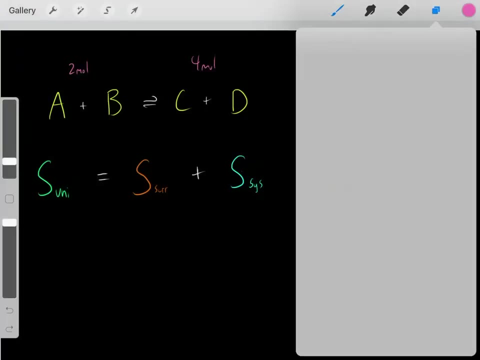 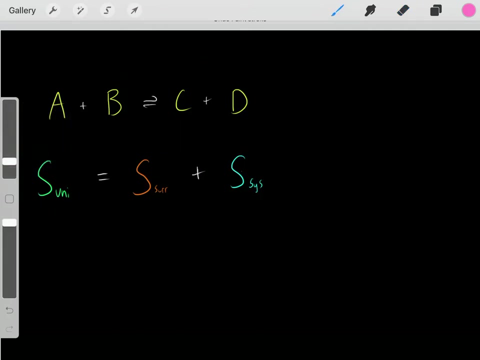 then we determine how the entropy of the universe changes And then we know that if overall this was higher than that, then we can determine how the entropy of Böylevariée reached. Pa text to understand how term ceremonies were planed came out a little bit farther than pause. rolou will always stay, but then I was too lazy to plain her mind, if you. 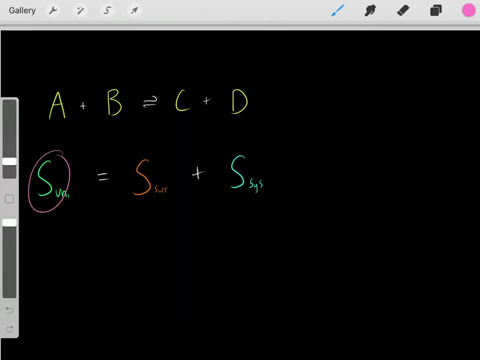 came out premature on me for that it was too long. So you don't just look at the moxibustion mediation: spontaneous. If this reaction occurred and the entropy of the universe increased, we know this reaction is spontaneous. So this is one way you can look at it. but there's another way you can. 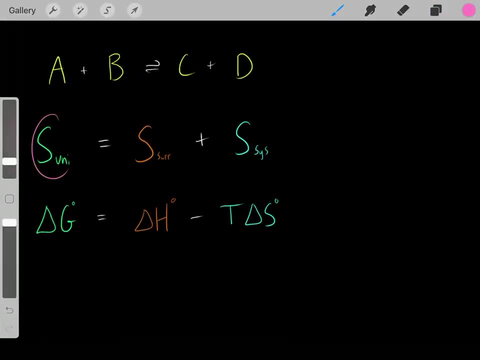 look at this Again. you can determine the entropy of the universe, how that increased. and if the entropy of the universe increases, we know the reaction is spontaneous. But another term that tells us the exact same information is this Gibbs free energy term. They essentially represent the 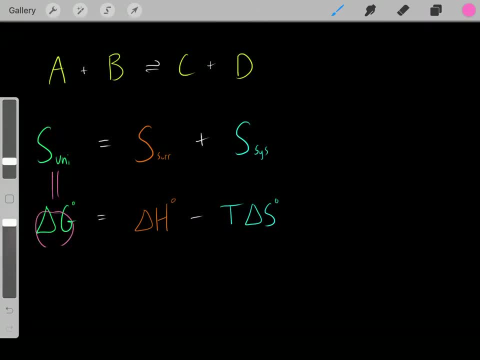 exact same thing. They're identical. They're just different ways of looking at the exact same thing. And we know: when the entropy of the universe increases, that's spontaneous. But with Gibbs free energy, when the Gibbs free energy decreases, that's spontaneous. So when looking at this, 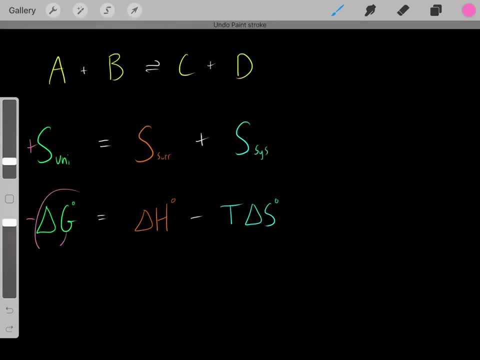 reaction if the Gibbs free energy decreased. we know that's spontaneous, But again they tell us the exact same thing And just based on the sign conventions that humankind has decided to use. negative delta G is spontaneous, but positive entropy is spontaneous, But again they represent. 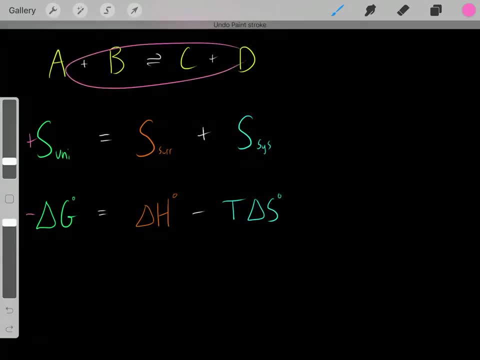 the exact same thing, And again the entropy of the system can also be used to determine the represented by this delta S, which again represents the entropy of the system. So again they represent the same thing And again remember the entropy of the surroundings. How do we know? 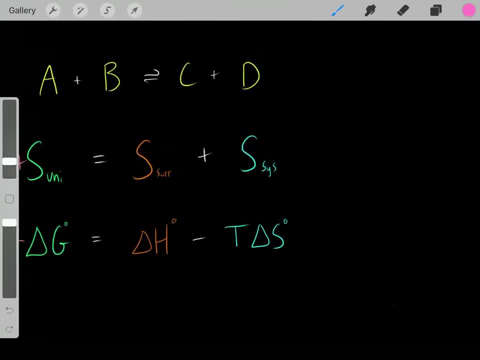 the entropy of the surroundings changes or increases or decreases. Well, we know, if it's an exothermic reaction, that the entropy of the surroundings increase. If it's an endothermic reaction, the entropy of the surroundings decrease. So therefore, we know the entropy. 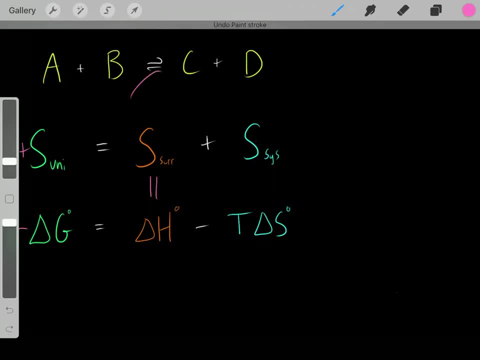 of the surroundings is directly related to whether this reaction is exothermic or endothermic. So that's another way. Instead of focusing on the entropy of the surroundings, we can look at the seeing how the entropy of the surroundings changed. we could just focus on if this reaction 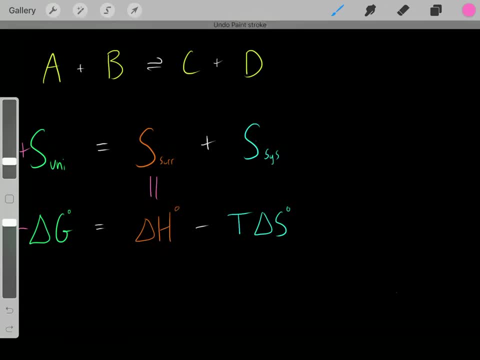 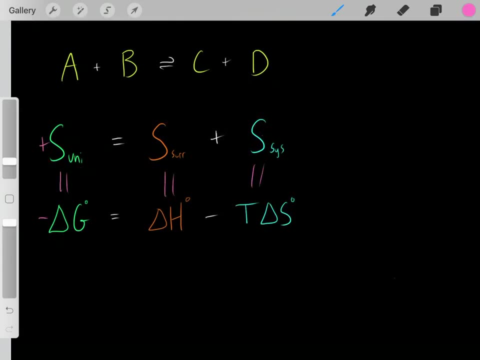 was endothermic or exothermic. And again they tell us the exact same thing. They represent the exact same thing. So there are these two equations which essentially are parallel. They all mean the exact same thing and they're telling us the exact same information In just the convention that. 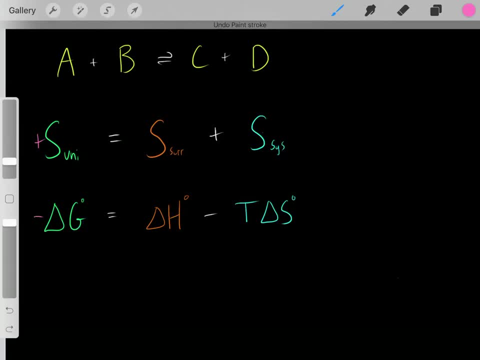 humankind has decided to use. we decided that let's just say that a negative delta G is spontaneous and represents an increased entropy. So therefore, we know negative delta G is spontaneous. So therefore, these terms, if they create a negative delta G, that's thermodynamically, 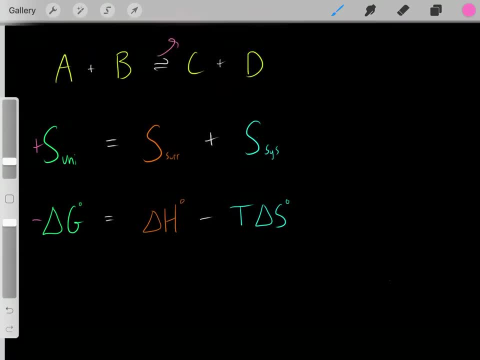 favorable. And again, so that makes sense, because we know an exothermic reaction has a negative delta H which, again we said, is spontaneous, because a negative delta H promotes a negative delta G, which is spontaneous. So again we said that if endothermic or exothermic, and again, 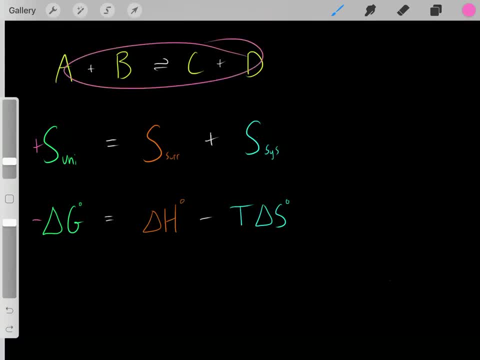 if this reaction was endothermic, it required heat. that's a positive delta H. That's a positive delta H which would promote a positive delta G, which is not spontaneous, because we said a negative delta G is spontaneous. So again, these two terms tell us the exact same. 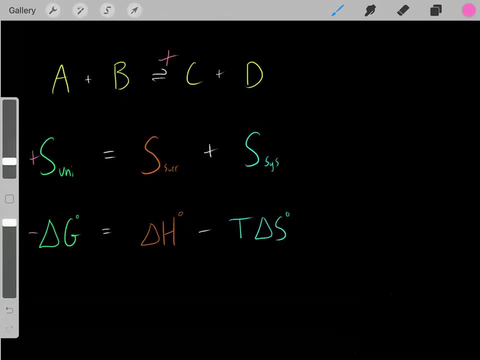 information. And again we said if the entropy increased, that spontaneous of the system, and again because we have a negative sign here. so we know if the entropy of the system increased and became more positive, so this entropy of the system became more positive because it's negative. 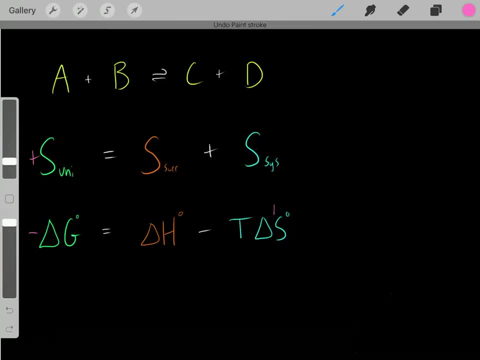 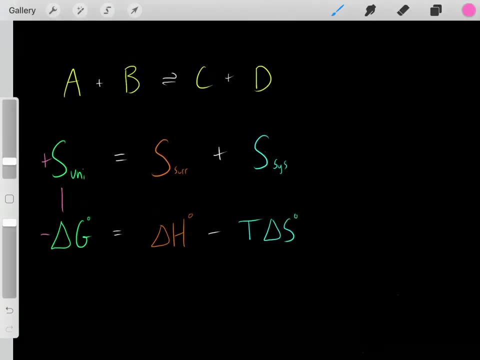 that will create a negative delta G, which is spontaneous And again, so that makes sense. So again, I know the sign conventions are confusing and it's a little arbitrary, but it's just something you need to be familiar with. But these 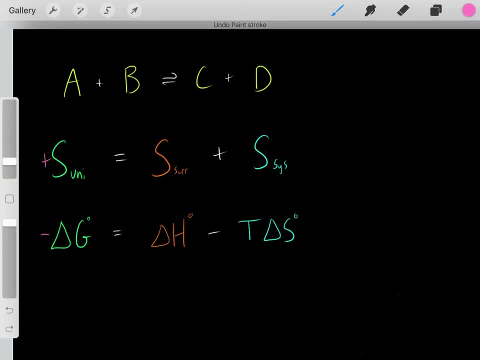 terms essentially represent the exact same thing, And also the entropy of the system. you have to multiply by the temperature of the system, And the way I like to think about this is the entropy of the system. how big of an impact it has on the delta G depends on the 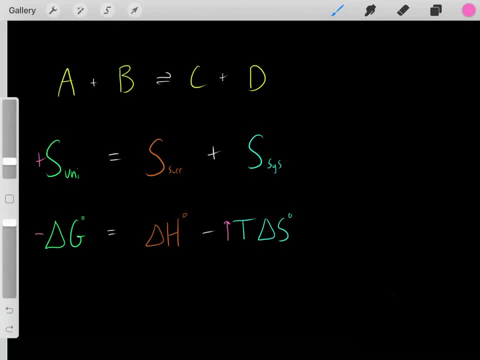 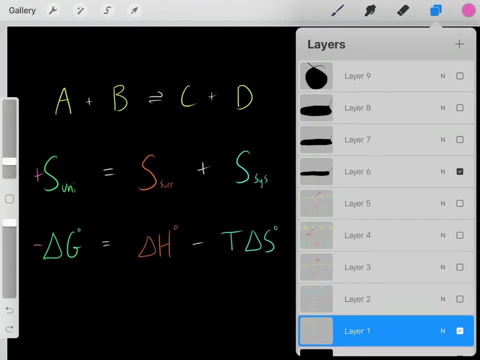 temperature. The higher the temperature, the bigger the impact the entropy of the system has on this delta G. So that's just something you need to be familiar with, But again, so let's do one last example. Let's say we had this chemical reaction: 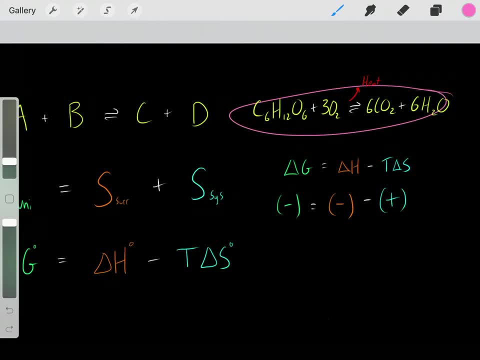 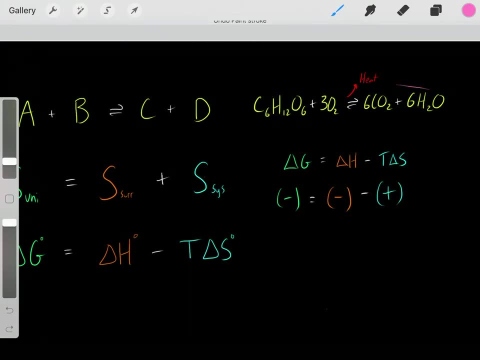 Is this reaction spontaneous? Well again, we know. if this reaction leads to the entropy of the universe increasing, we know this reaction is spontaneous. But another way you can look at it is determine if the delta G of this reaction is negative. If this reaction has a negative delta G, we know that's spontaneous. 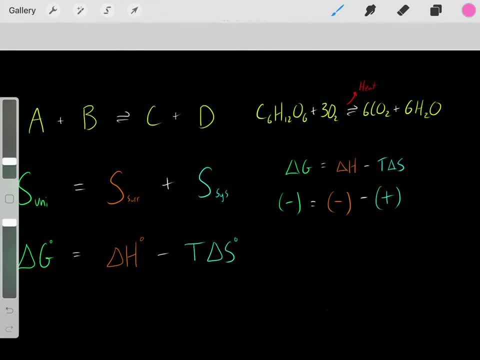 So how do we determine the delta G of this reaction? Well, again, if we know the enthalpy of this reaction, that's one thing. So, again, we said, this reaction released heat. This reaction released heat, so therefore it's exothermic, so therefore it has negative delta H. 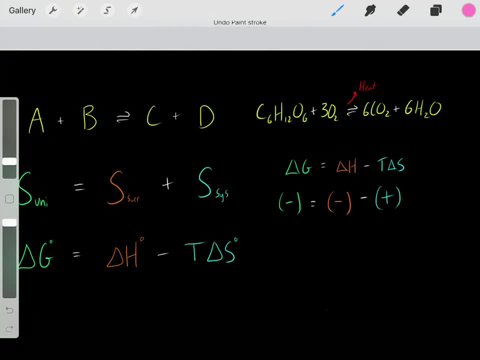 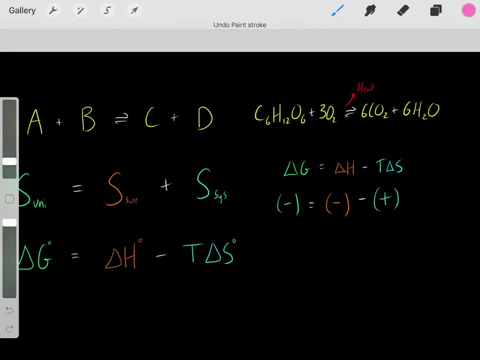 This would have negative delta H. So again that's favorable because that promotes a negative delta G, so that promotes spontaneity. And again we also saw we had 4 moles to went to 12 moles. So we know the entropy of the.